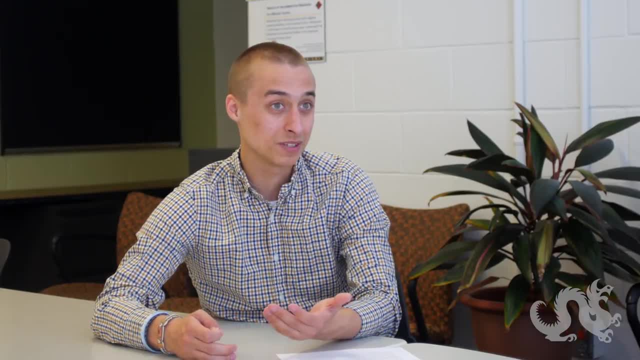 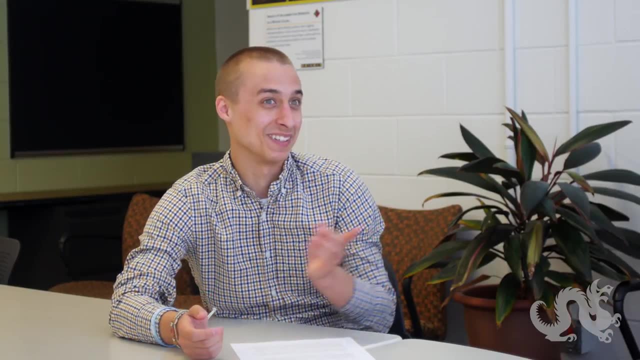 of using wet lab. Yes, going through classes you sometimes get some lab experience, but being fully immersed and like this is all I did for the six months was awesome And I was able to put my input out, there be like I did that, like it was awesome seeing that. And then for my second co-op, I worked. 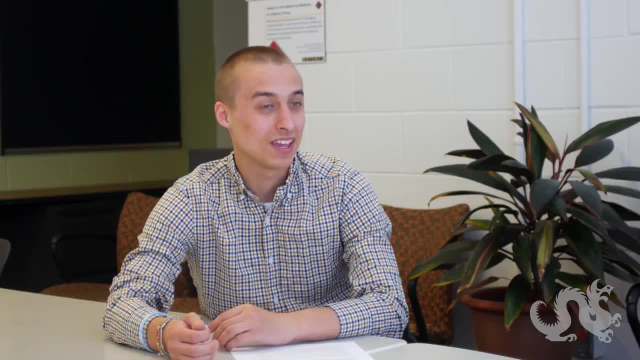 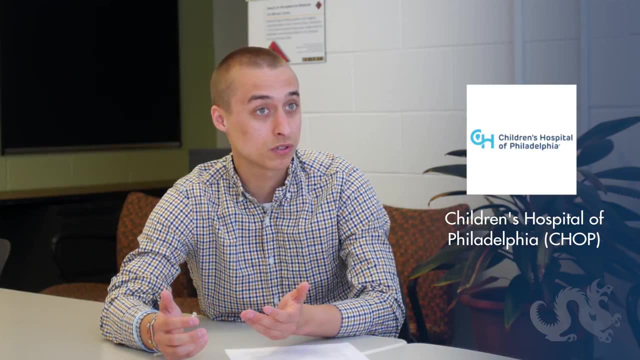 at over here at Children's Hospital Philadelphia, also known as CHOP, and I was doing clinical research in their plastic and reconstructive surgery department, Mainly working with those with congenital craniofacial disorders- cleft palate, BPD, cleft lip. 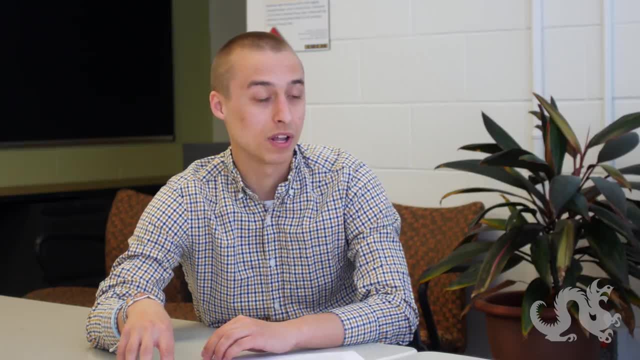 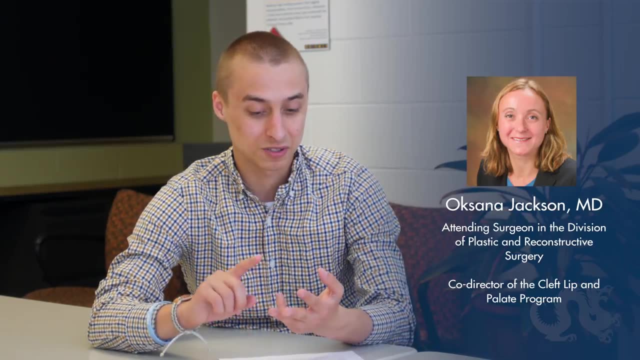 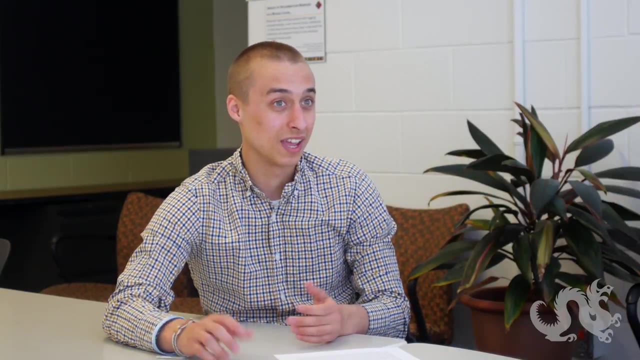 and I specifically worked under Dr Jackson, Oksana Jackson, But I also got to work with Dr Swanson, Dr McGee and a whole bunch of other surgeons, doctors, nurses, psychologists, the orthodontist and the research team. I got to sit down in the touchdown zone where all the surgeons sat, So 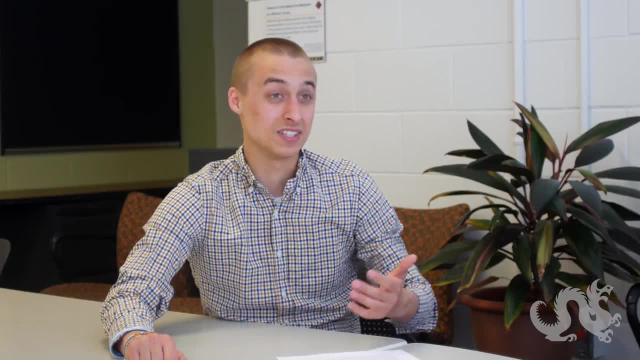 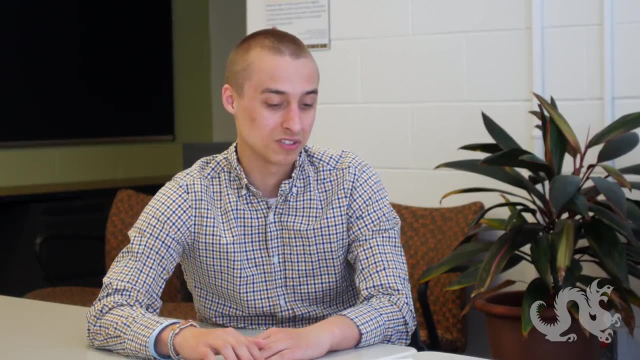 when they had their lunch. I was sitting there listening to the conversations that they had, getting to see cases that they had that weren't with some of the children because they worked at other hospitals as well- Asking questions whenever I needed them. So one of the surgeons- 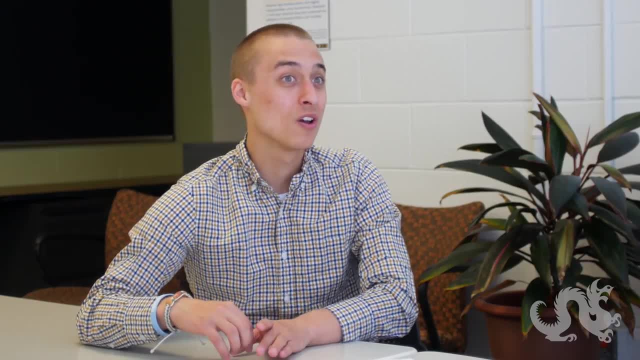 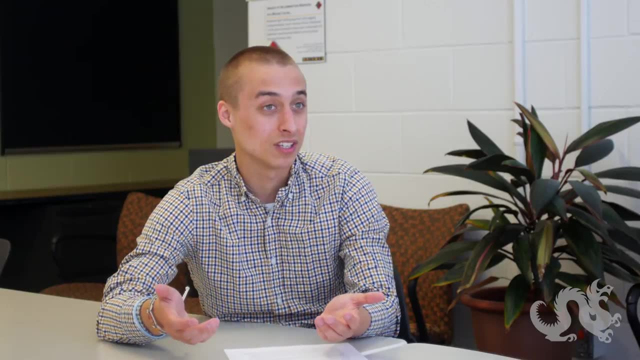 he's a medical illustrator and he drew out for me the different deformities, the way they would proceed in surgical procedures, and 10-15 little notes. So I got to go in with a computer and talk to the kids and record speech for them, Then get consent for a research database that we're doing. 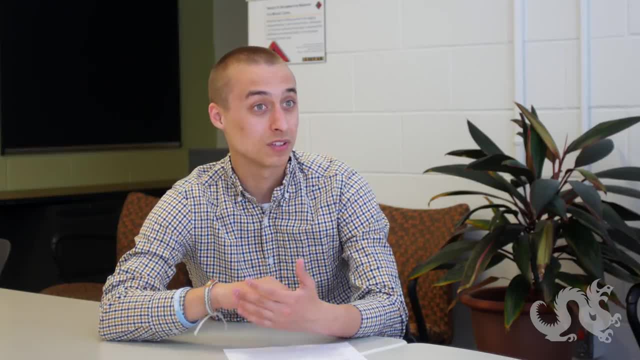 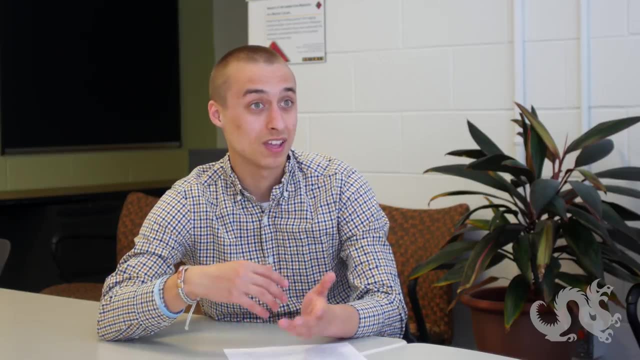 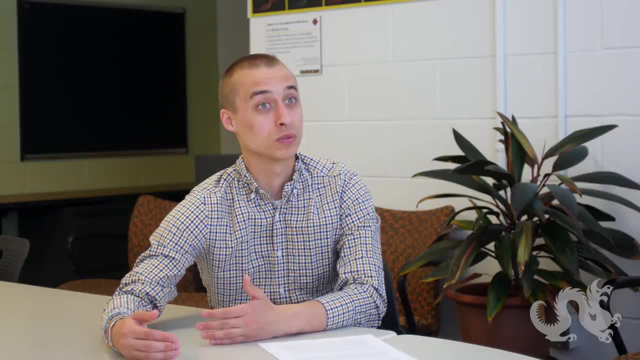 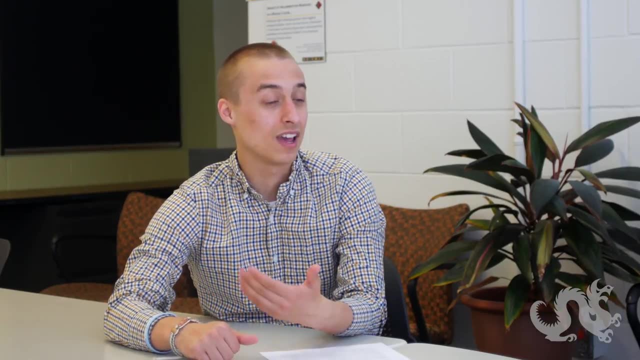 It was a lot of fun. It was a lot of fun. They hadn't though this clinical research so I knew there was going to be projects. They weren't sure really what was going to be on the table when having the job. As more projects came in, we just didn't work With that. they 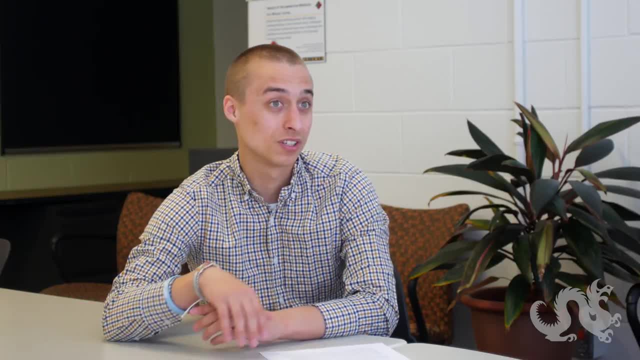 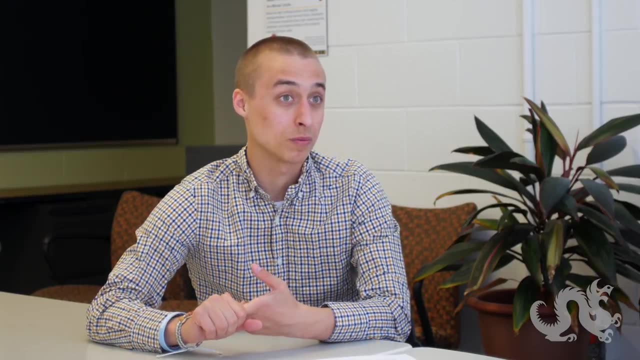 had the implication of possibly getting published, of which I've been told, once it gets published, that we're on a paper, which is a huge leg up. I got connections for possible recommendations for medical school. I asked if I could go and see the OR, so I got to see some surgeries. 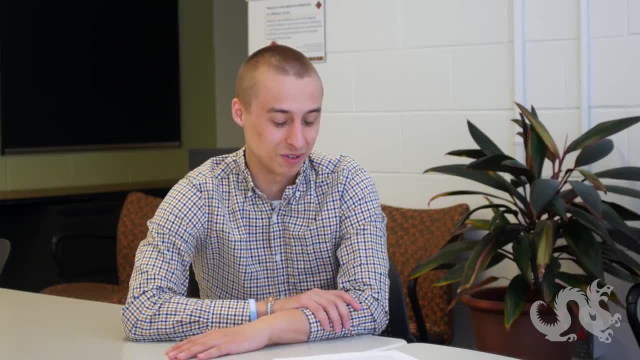 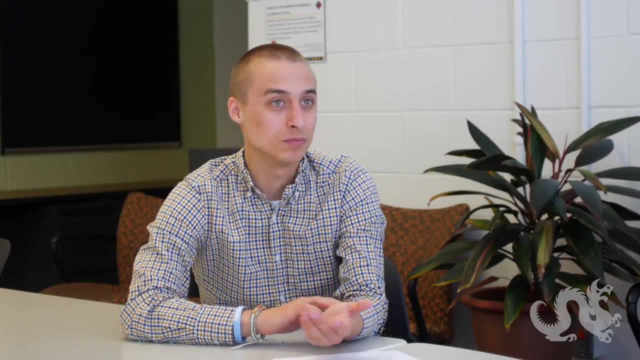 which is what I want to do in my life. so I invented that more so, And I got to go to the ER. I got the shot on the ER during nighttime hours, so doing like a 8 pm to 1 am shift or 6 pm to 1 am. I was there one time. 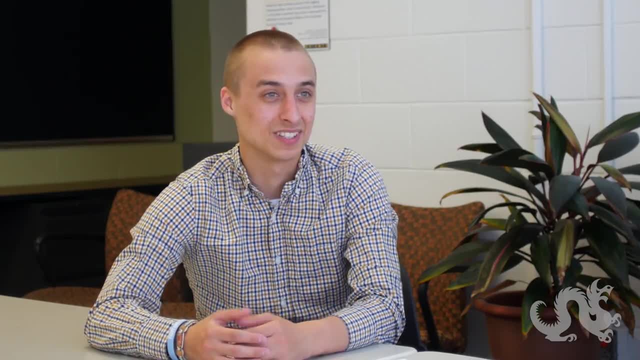 And you can see the wide range of cases. It's just you can't do anywhere else. 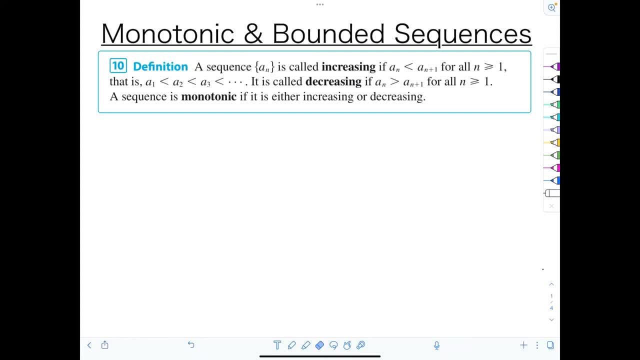 Welcome to Mac TV with Professor V. In this video, we're going to look at monotonic and bounded sequences and, in particular, how to determine if a sequence is monotonic and if it's bounded. Well, definition: what does it mean for a sequence to be monotonic? Definition. 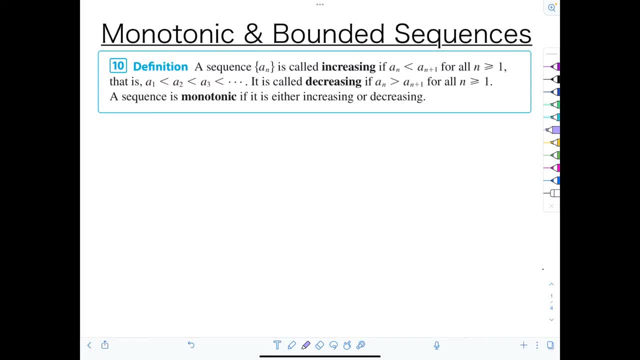 is as follows: A sequence: an is called increasing if an is less than an plus one. So an plus one would be the term that follows an for all n greater than or equal to one, That is, a1 is less than a2, is less than a3, etc. A sequence is called decreasing if an is greater than an.